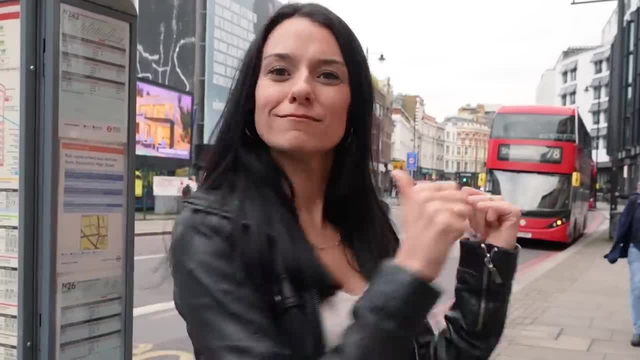 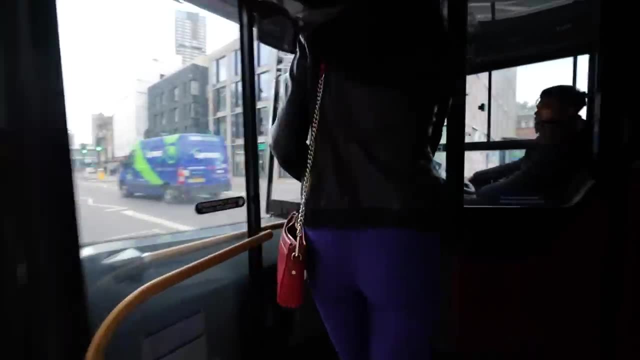 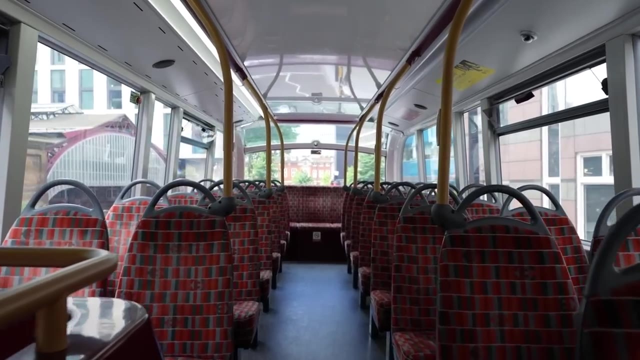 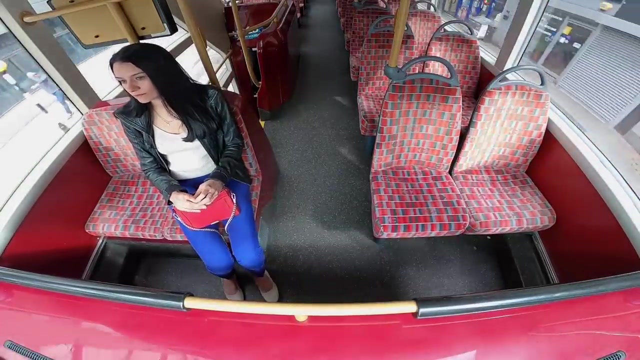 around this city. And the first option is right behind me: Let's go In London. we have the very famous double-decker buses, which are actually the cheapest way to get around London. I think they're a little bit more comfortable too, and the best part is that if you get a front seat on the top. 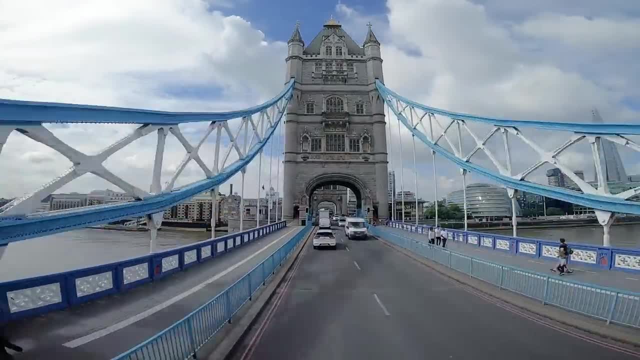 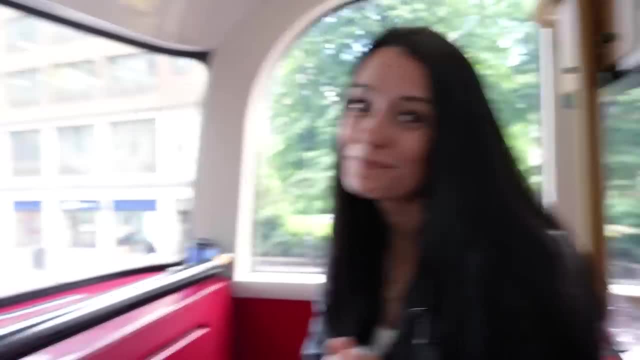 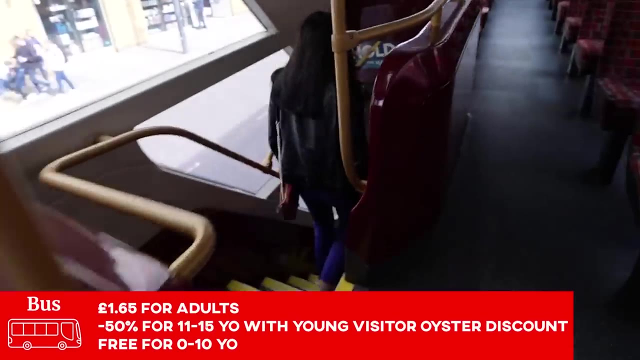 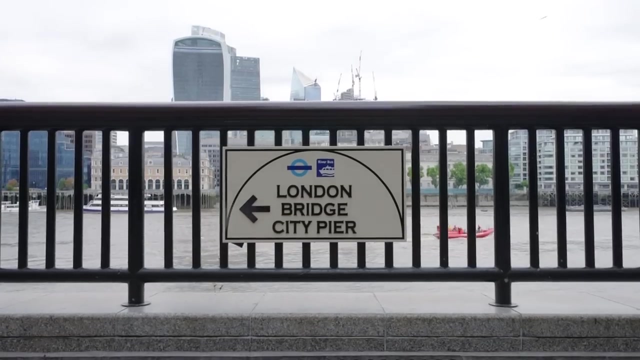 deck. your views are amazing. The downside of buses, though, is that they get stuck in traffic, so it can actually take you a really long time to get some places- sometimes Happy- on a bus. Yeah, Our next motor transport is right here. We're going to go down to Canary Wharf. 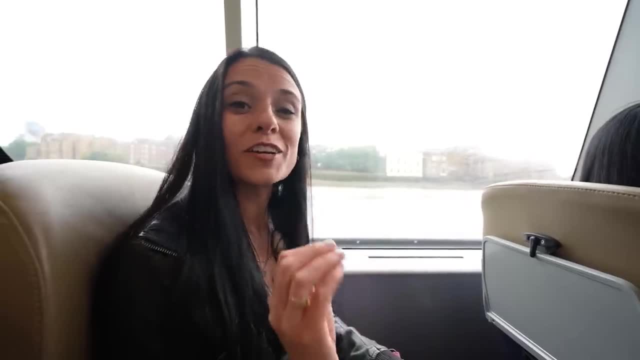 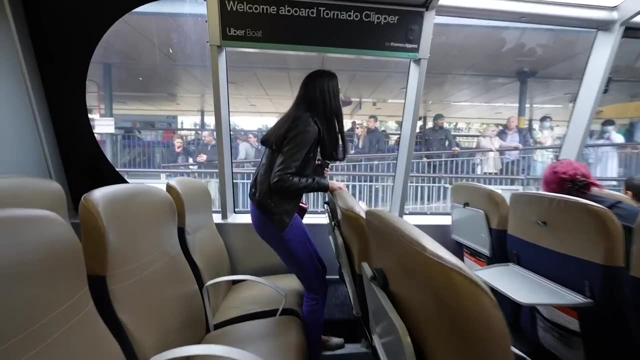 We're on the river bus- another bus. This is a public transportation option here in London. There are 24 different piers where you can get on the river bus, and the price that you pay for your journey depends on how many zones you travel through. There's three of them. 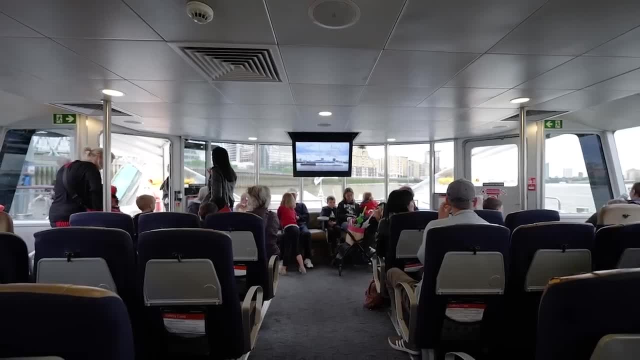 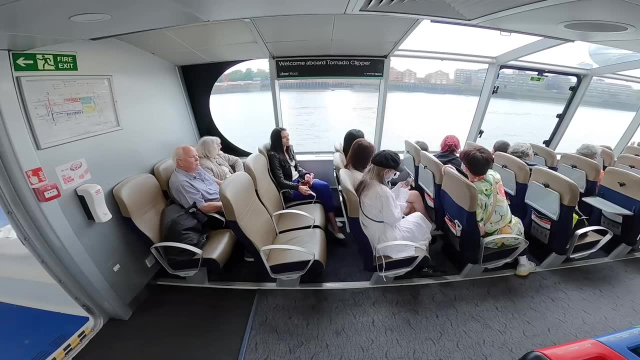 central, east and west. The boat is actually really nice. There's even a cafe on board and a toilet. It's actually a really comfortable way to travel around London if it works out for your route, but the downside is it's probably the 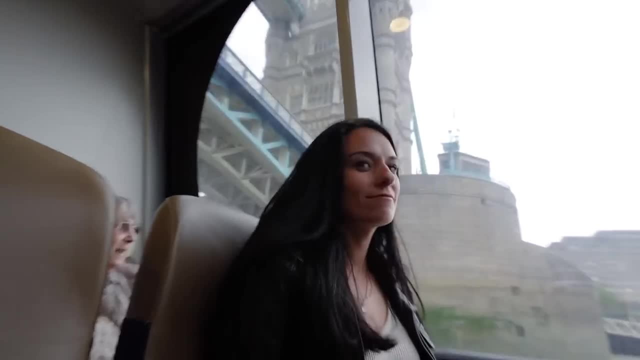 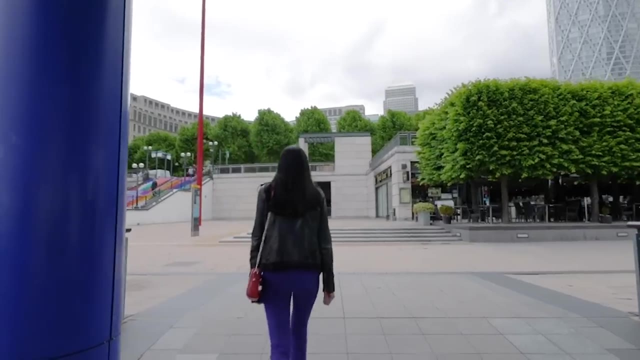 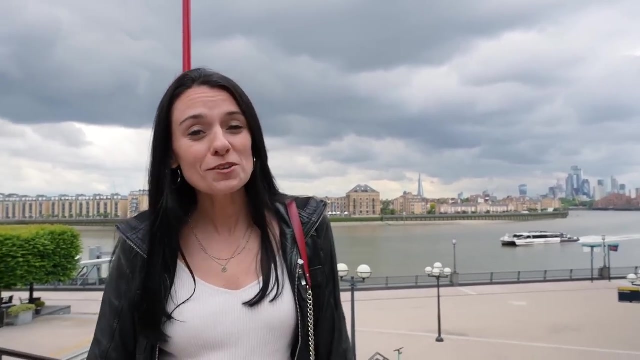 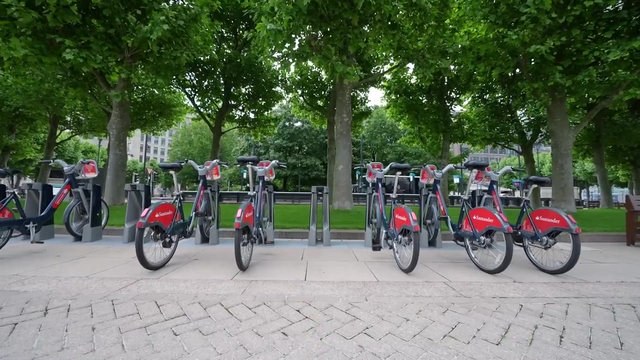 most expensive way to get around London besides taxi. This is pretty cool. We made it to Canary Wharf on that type of boat and our next motor transportation is right over there. These are Santander bikes, sometimes called forest bikes, and this is the city's public bike system. There are 12,000 bikes. 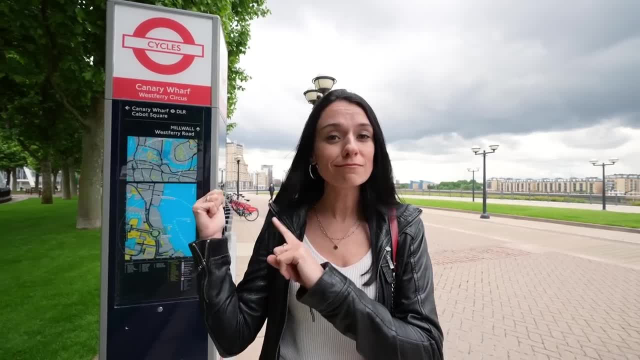 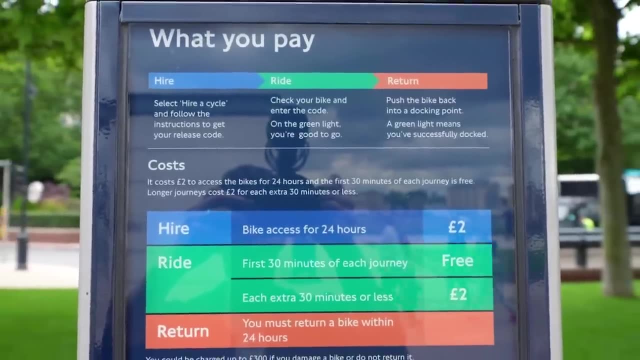 around the city and 800 docking stations, including this one. The cost of using these bikes is a little confusing, So hear me out. First, you pay two pounds for 24-hour access to the entire bike system, no matter how many bikes you take out. Then, for each bike that you take out, 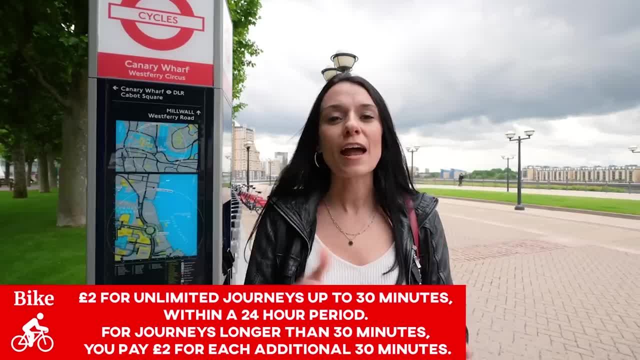 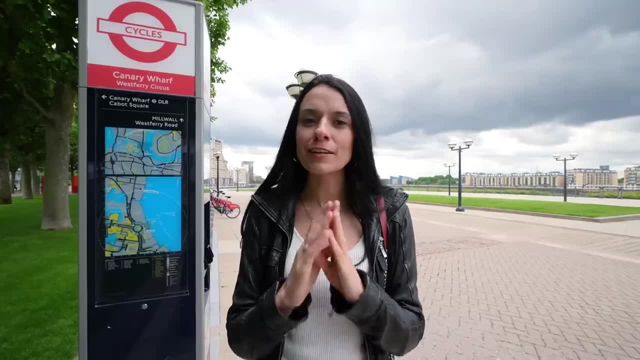 your first 30 minutes of using it is completely free, and for every 30 minutes after that you will be charged an additional two pounds. For tourists. it can be tricky to cycle around London and a little bit intimidating, so if you do want to cycle, I recommend getting the bikes at one of our many major parks. 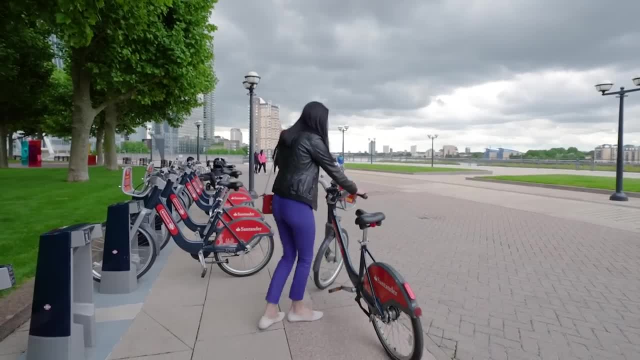 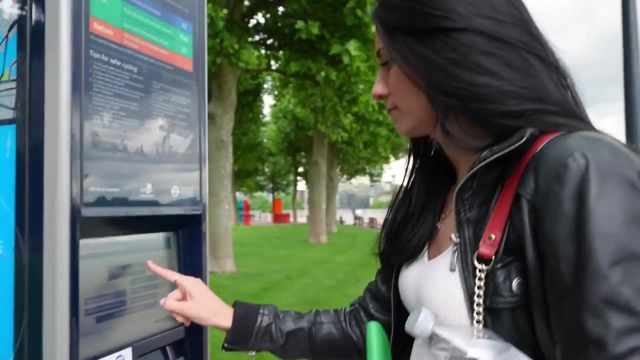 around the city, like Victoria Park or Hyde Park. It's very fun to cycle around them and it's a lot of fun. You get to see a lot more of the park on two wheels. This is the docking point. we're gonna get two bikes. 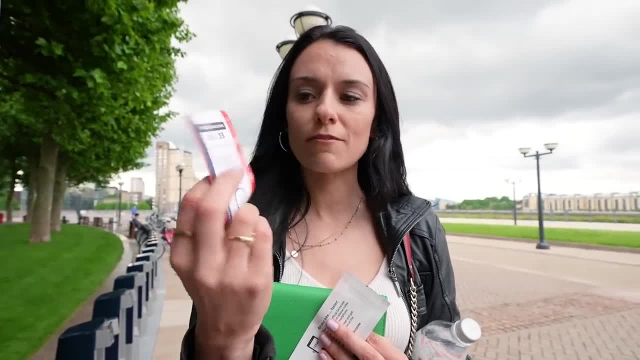 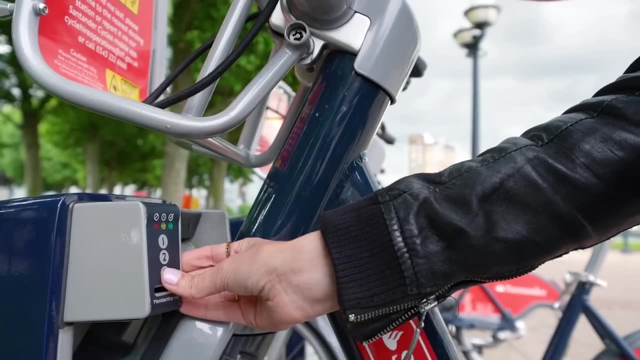 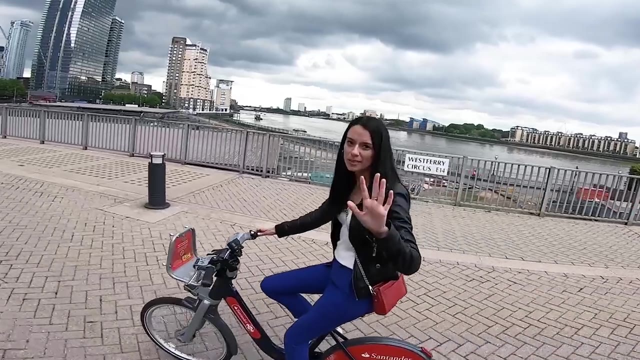 So when you rent a bike, you get these printouts that have a code on the top and that is what you type in to pull out one of the bikes. Let me show you, Bikes are super easy to get. I do have a full video that I've 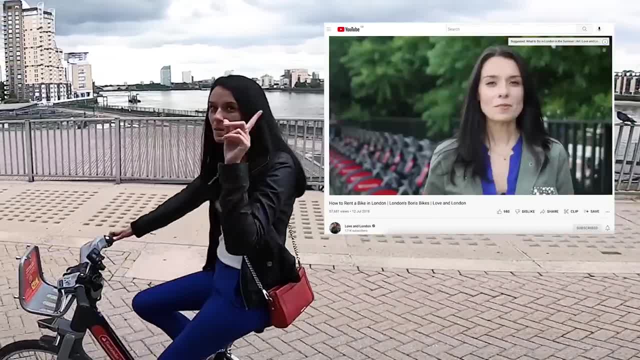 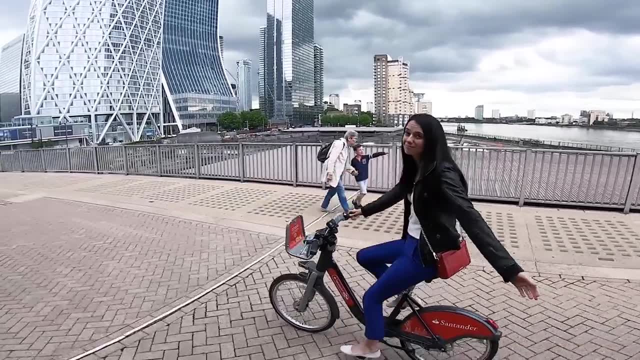 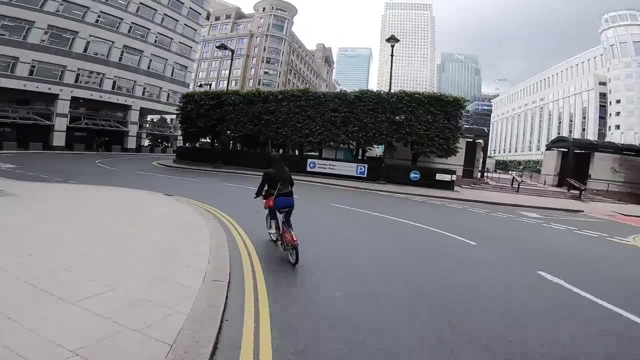 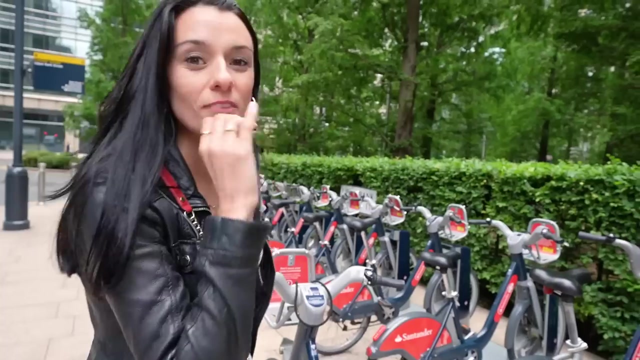 followed and can click the link on the top right here to get the. I have a full video that explains more about how to get them that you can watch by clicking the box popping up over here. but they are really fun and I just love exploring any city by bike. 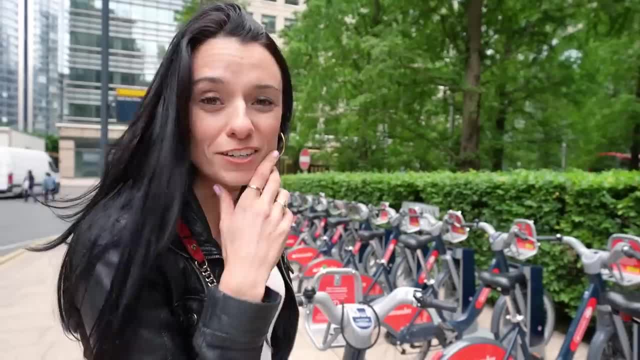 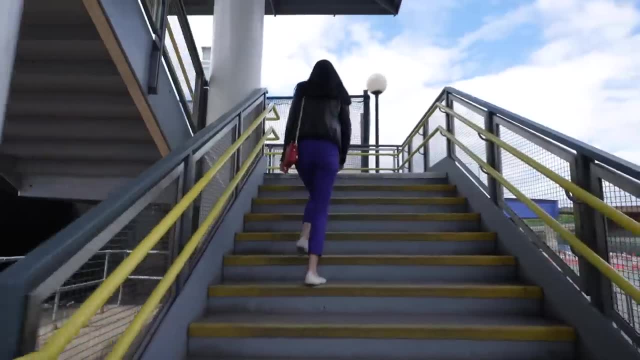 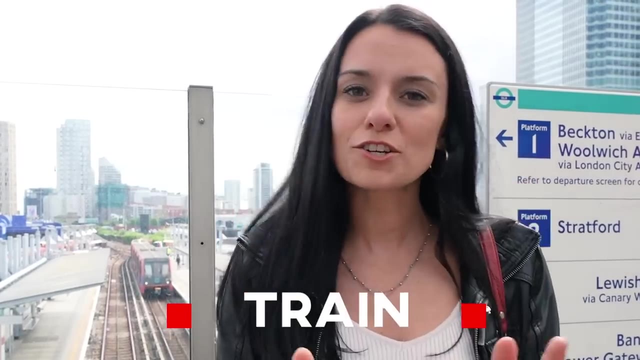 Let's do it wharf. this is like the financial district of the city, but we just happen to come over this way because of the boat, fyi. the next public transport option we're taking is the train. so in london we have the underground or the tube. those trains go under the ground, obviously, but we also have a. 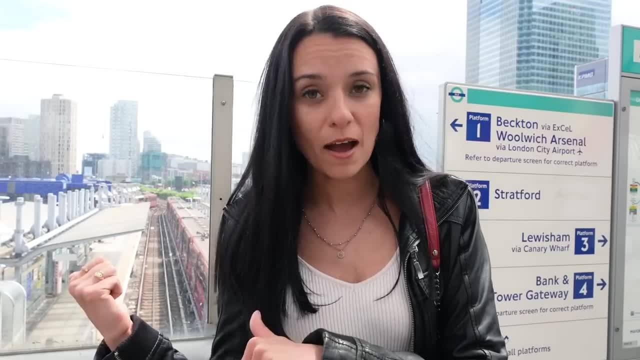 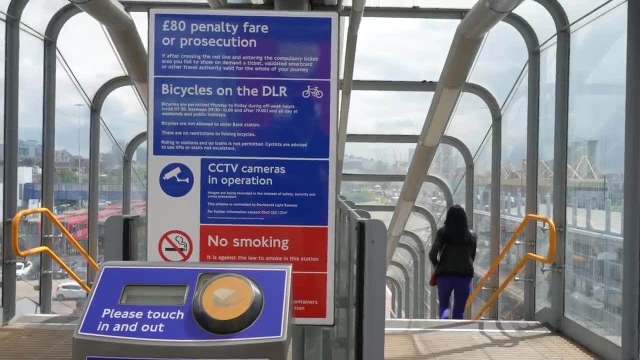 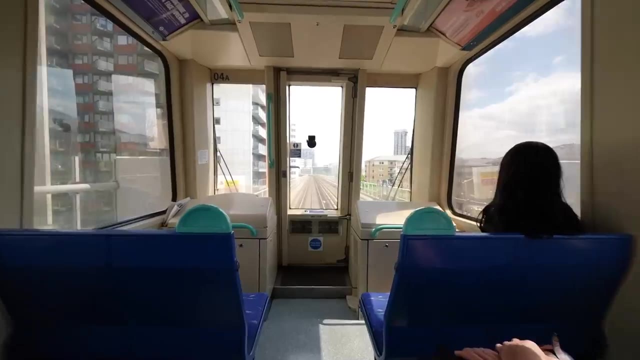 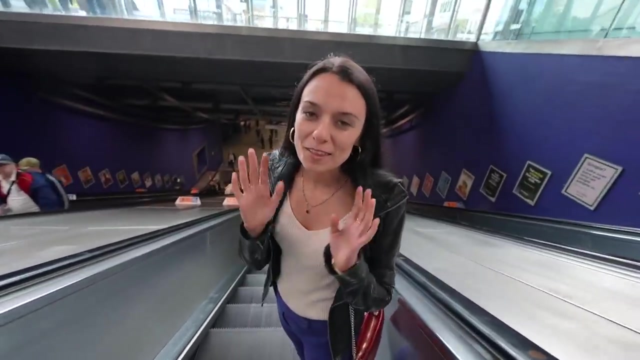 bunch of lines that are overground, like the dor, which is just behind me, and the actual line that's called the overground, so they're not as common for tourists to take, but you might end up popping onto one. we're about to go on the most popular transportation here in london, the underground. 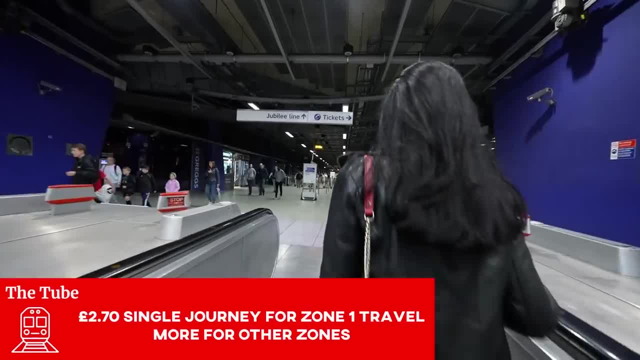 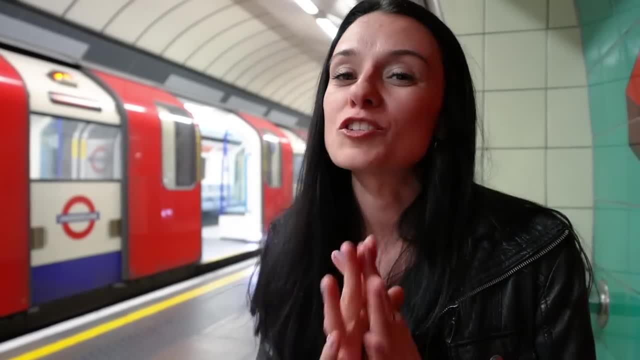 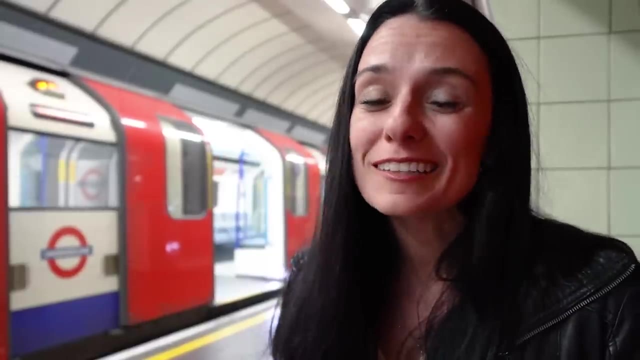 also known as the tube. there are 270 tube stations here in london and over 2 million people every single day take the tube system, and with 11 lines, you can get basically anywhere in the city on the tube. it's not all amazing, though. because the tube is so popular it gets really crowded, especially at